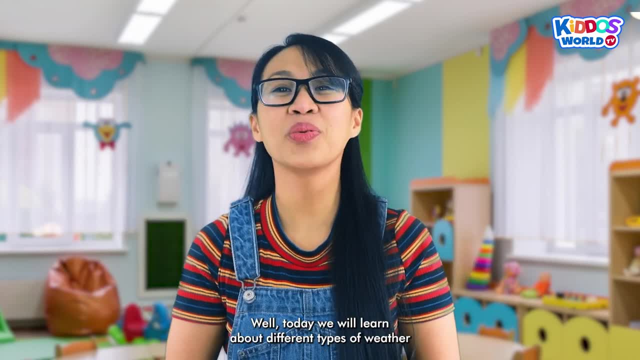 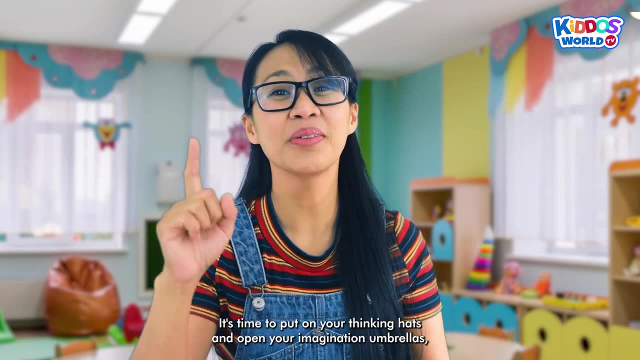 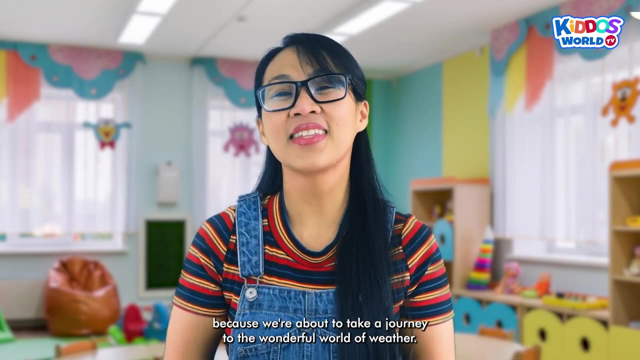 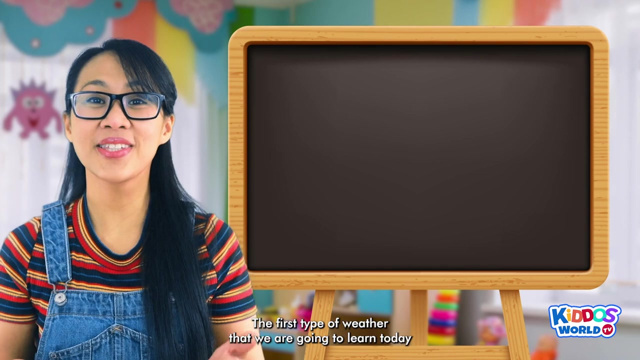 monster. Well, today we will learn about different types of weather and what makes them so interesting. It's time to put on your thinking hats and open your imagination umbrellas, because we're about to take a journey to the wonderful world of weather. Wow, The first type of weather that we're going to learn today is sunny. 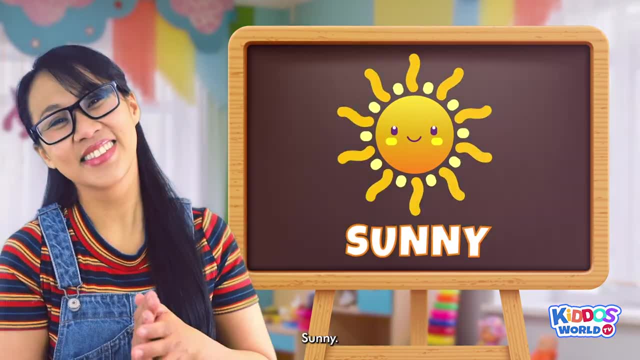 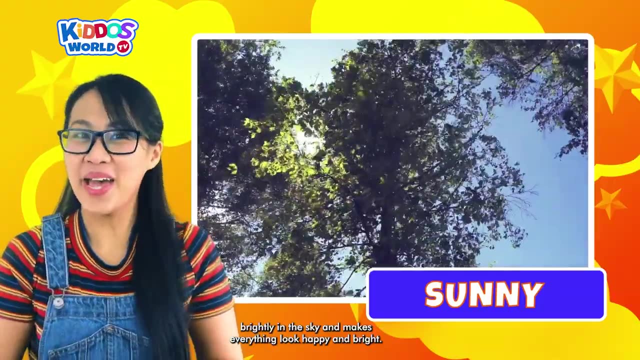 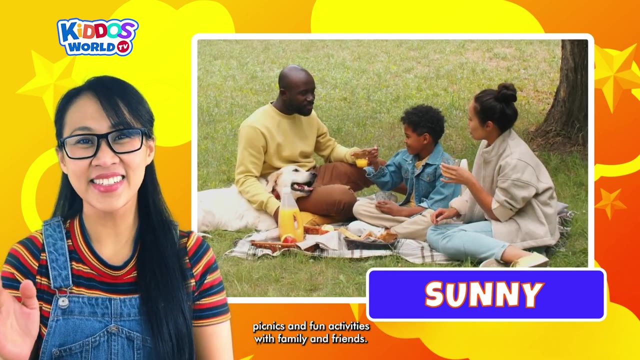 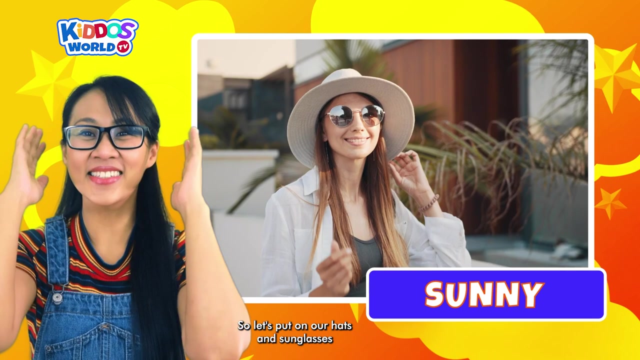 A sunny day is when the sun shines brightly in the sky and makes everything look happy and bright. This weather is perfect for outdoor play, picnics and fun activities with family and friends. So let's put on our hats and sunglasses and enjoy the sunshine. Let's 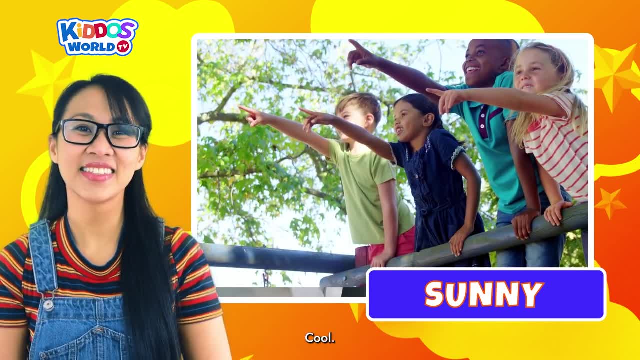 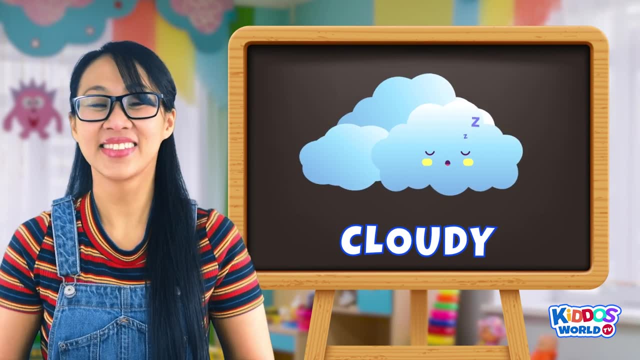 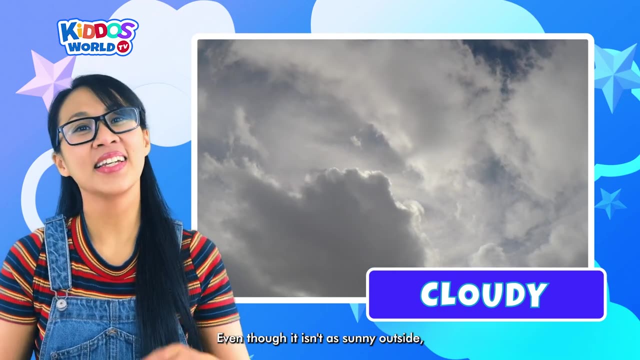 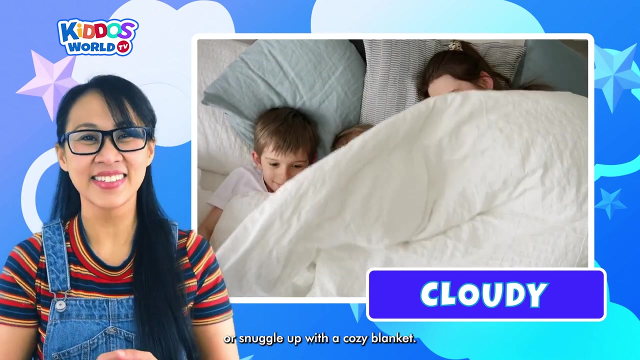 move on to the next type of weather, And our next one is cloudy. Even though it isn't as sunny outside, it's still a great time to play games, read books or snuggle up with a cozy blanket. Sometimes clouds look like animals or objects, if you're. 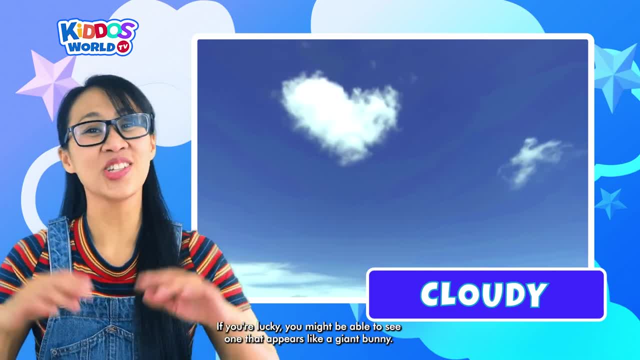 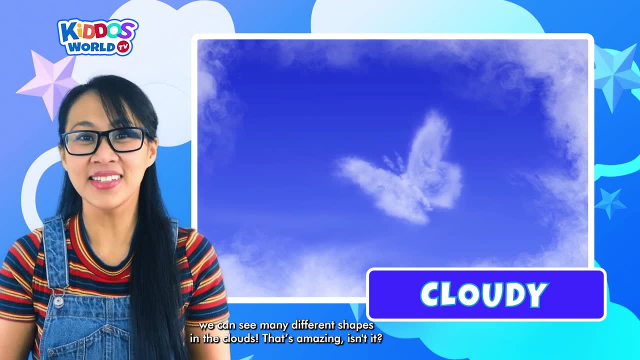 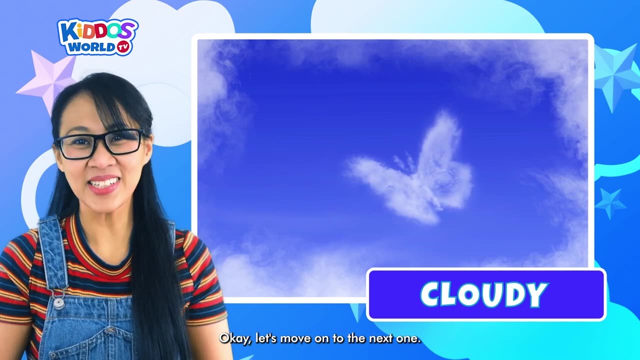 so lucky you might be able to see one that appears like a giant bunny. Using your imagination, we can see many different shapes in the clouds. That's amazing, isn't it? Yeah, Okay, let's move on to the next one. 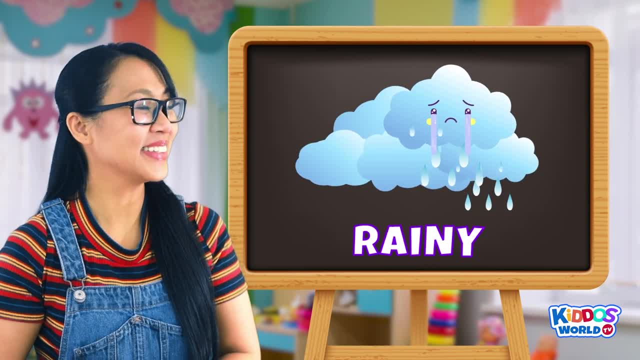 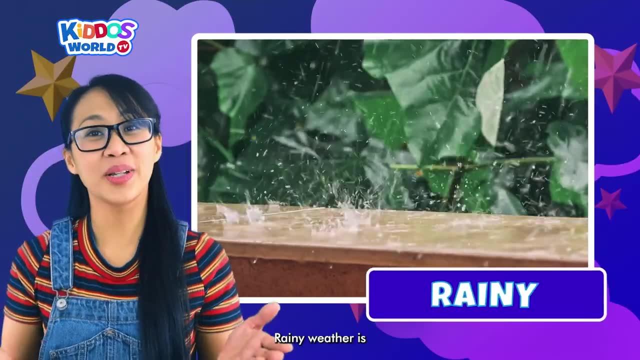 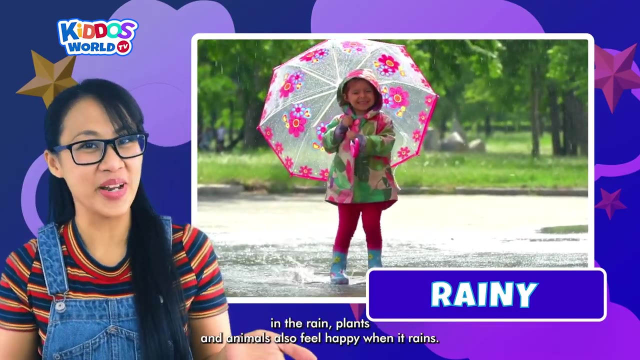 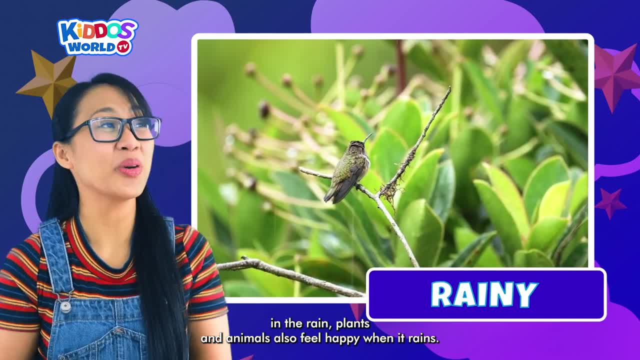 Rainy, Rainy, Rainy, Rainy, Rainy, Rainy, Rainy weather is when the sky tears up with joy. In the same way that we feel happy and want to dance in the rain, plants and animals also feel happy when it rains. Rain helps plants. 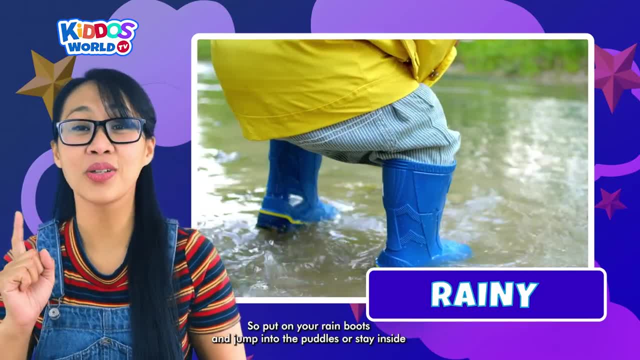 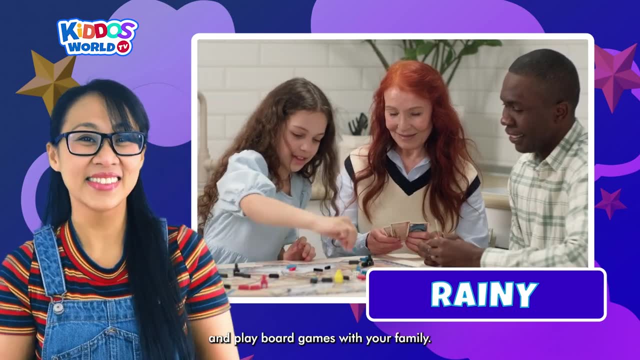 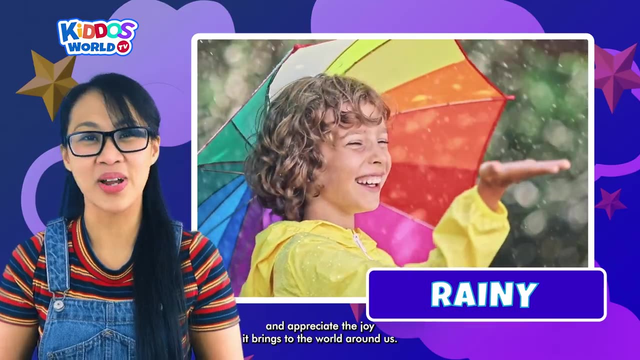 grow and provides water for animals. So put on your rain boots and jump into the puddles, or stay inside and play board games with your family. Therefore, let's enjoy the rainy weather and appreciate the joy it brings to the world around us- Wonderful. 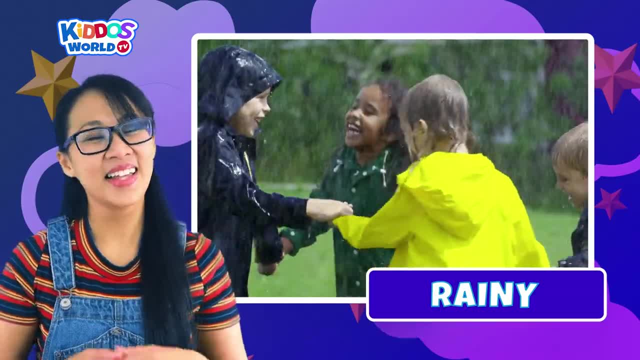 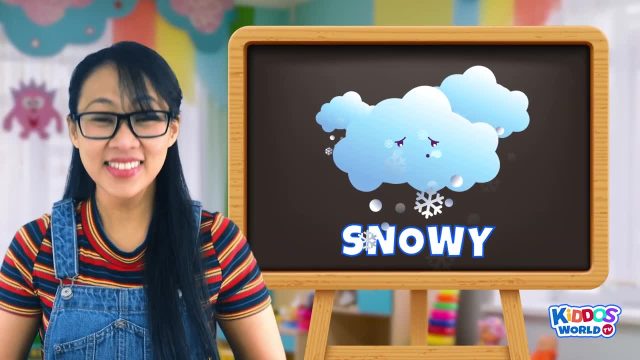 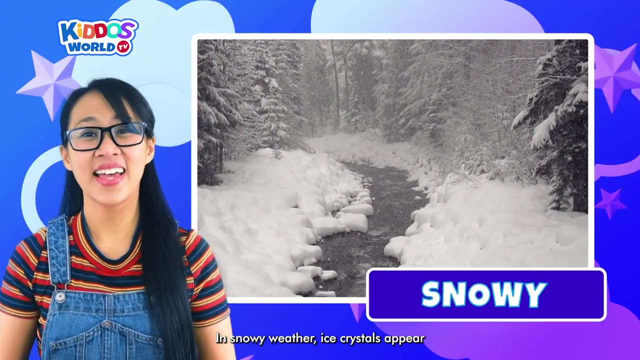 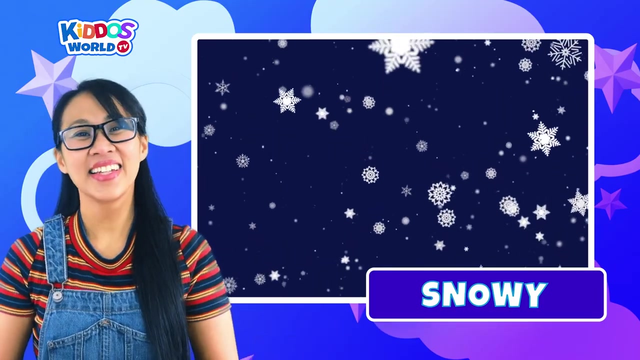 Wow, You're such an excellent listener. Let's learn more about weather types. Perfect, Snowy, Snowy, Wow. In snowy weather, ice crystals appear like magical snowflakes from the sky. Fabulous Like a cozy winter wonderland. snow covers everything like a white, fluffy blanket. 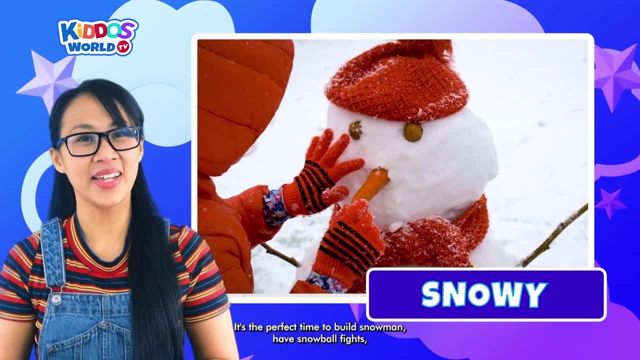 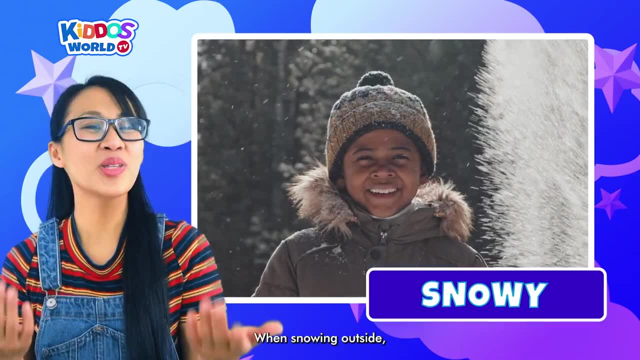 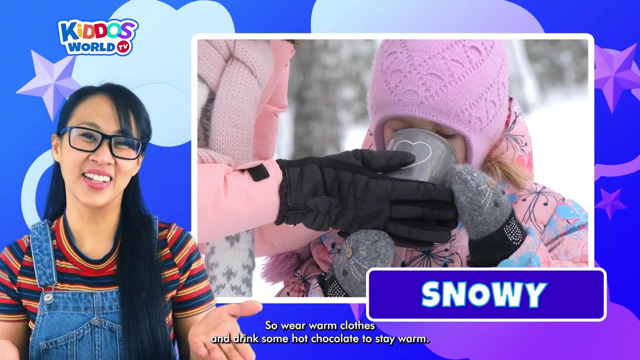 Hooray, It's the perfect time to build snowmen, have snowball fights or go sledding with your family and friends. When snowing outside it might be a little colder, so wear warm clothes and drink some hot chocolate to stay warm. 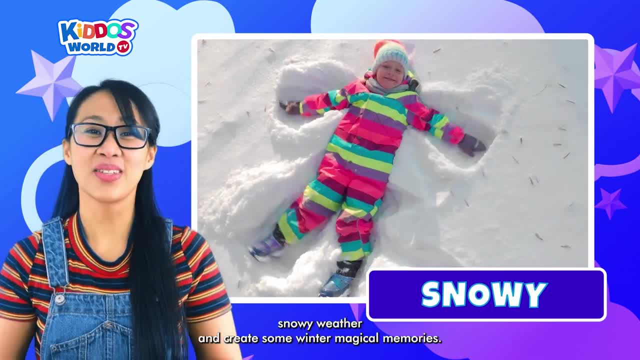 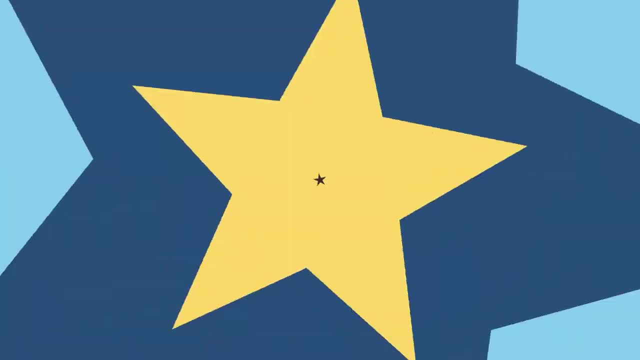 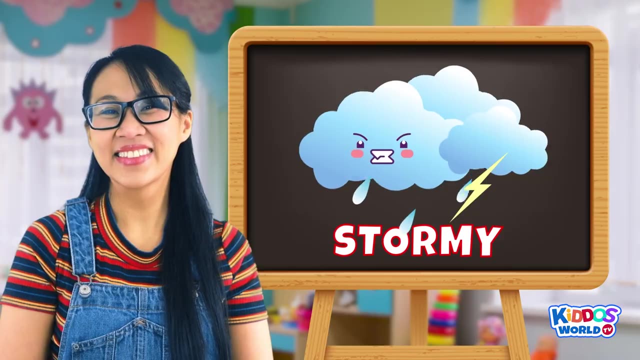 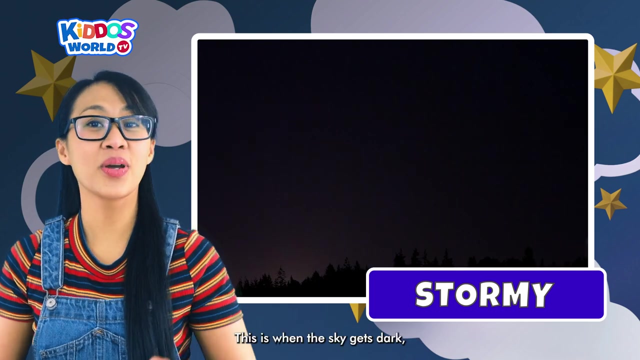 Love it. So let's enjoy the snowy weather and create some winter magical memories. How magical, right? Yes, Stormy, Stormy, Mother Nature puts on a show when it storms. Wow, This is when the sky gets dark: thunder, roars and lightning flashes. 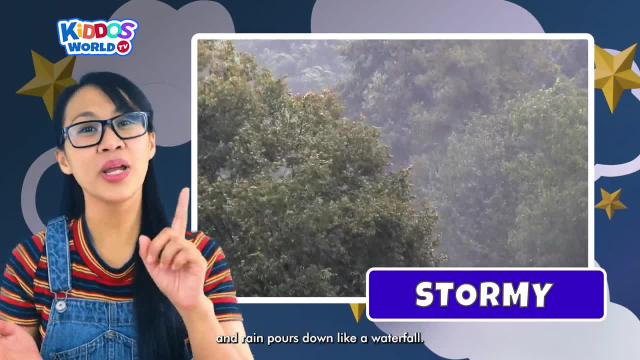 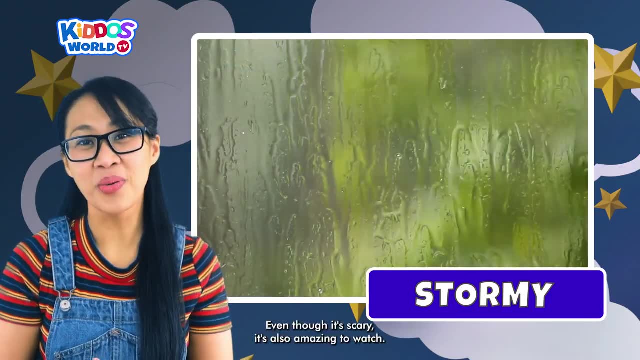 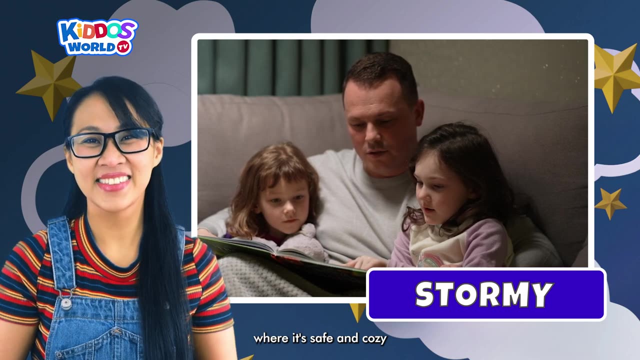 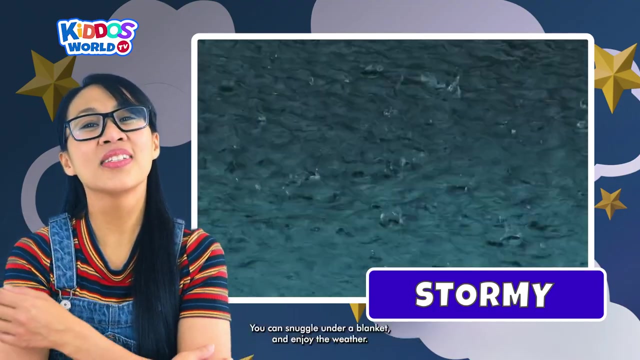 It can sometimes be windy and rain pours down like a waterfall. Even though it's scary, it's also amazing to watch. Stay inside when it's stormy. outside kiddos where it's safe and cozy, While reading books, playing games or listening to the rain and thunder, you can snuggle under. 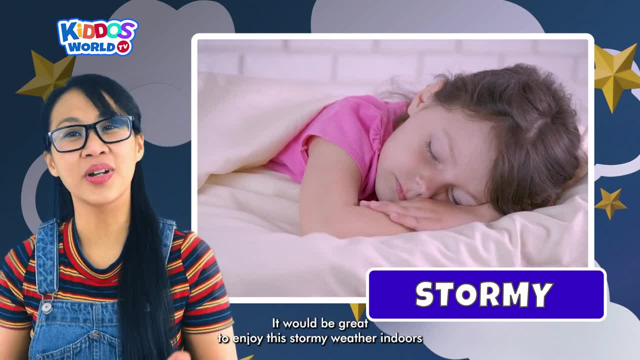 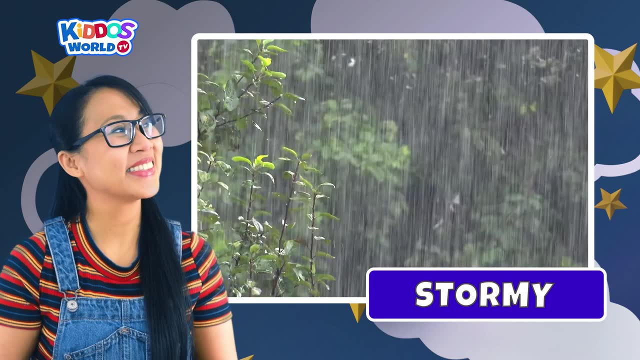 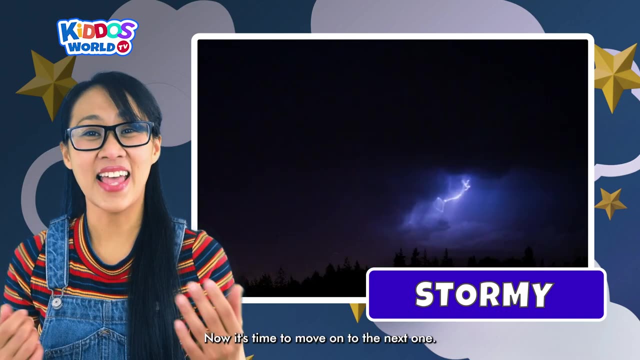 a blanket and enjoy the weather. It would be great to enjoy the stormy weather indoors and appreciate the beauty and power of nature. What a stunning display of Mother Nature. right kiddos? Yeah, Now it's time to move on to the next one. 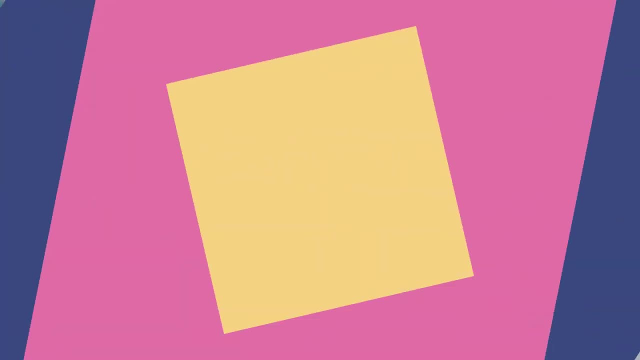 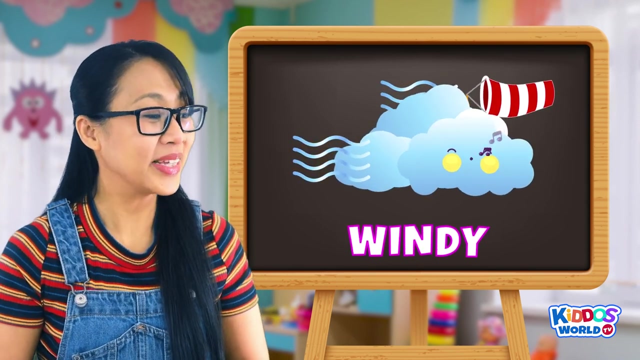 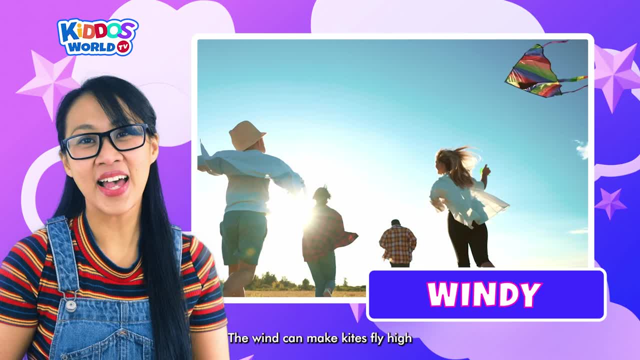 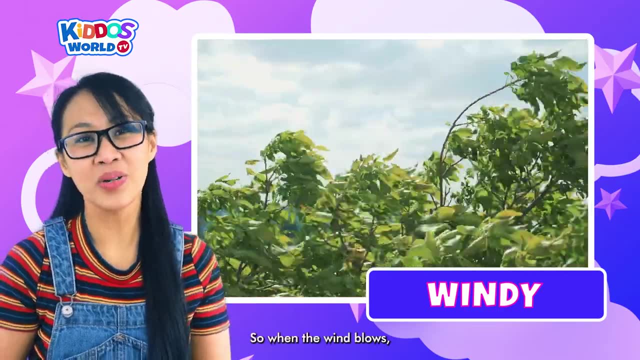 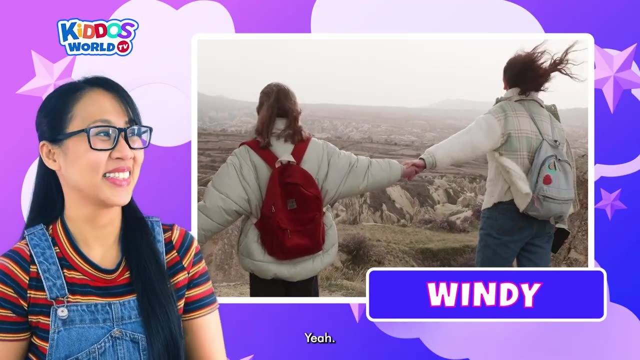 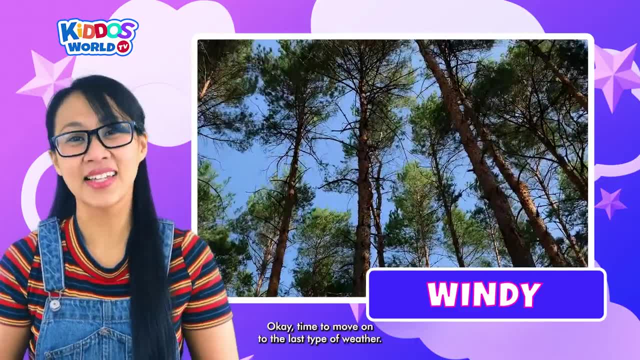 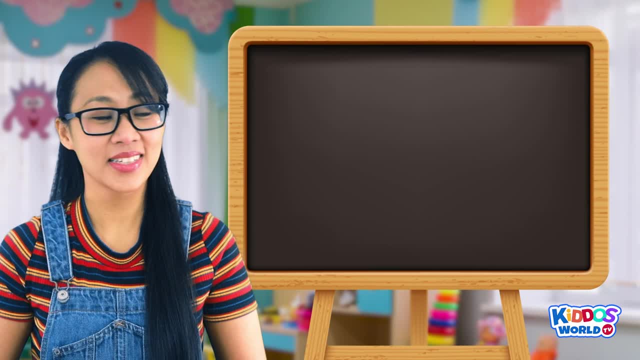 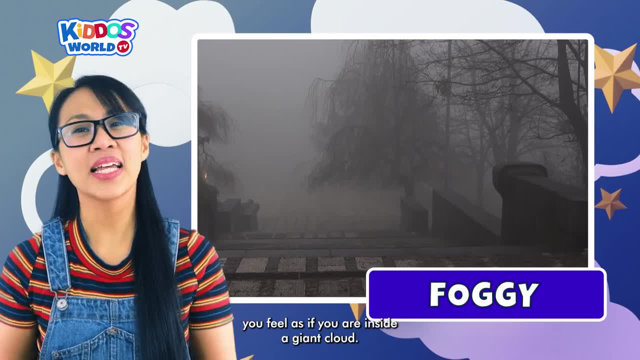 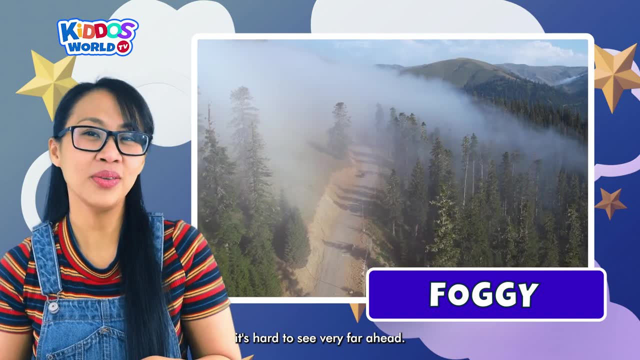 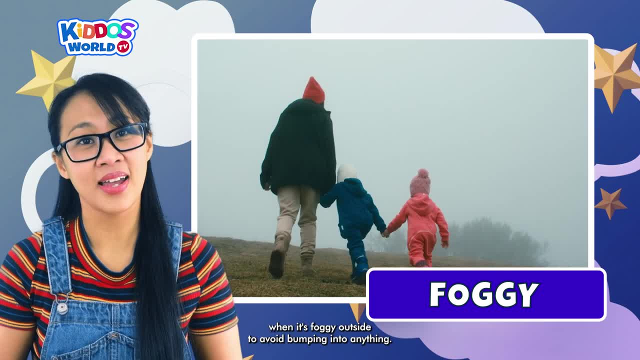 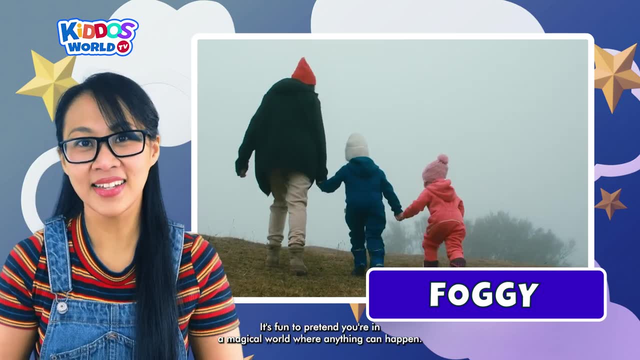 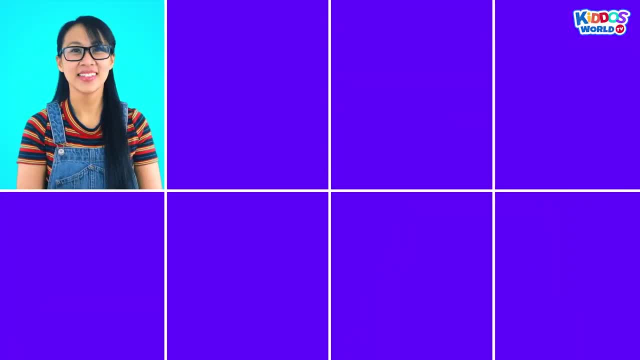 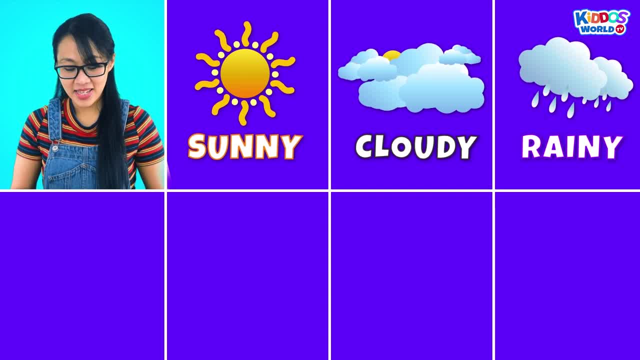 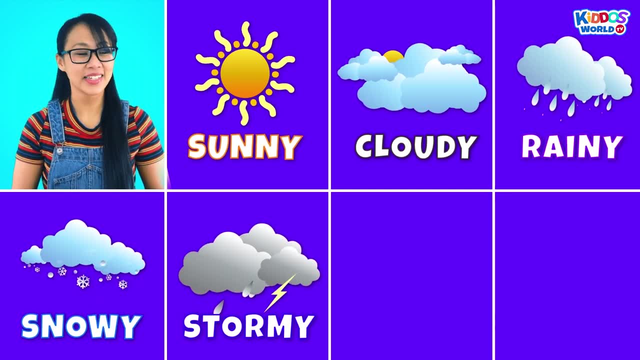 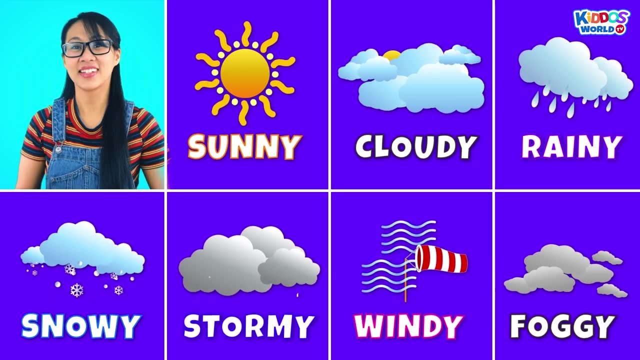 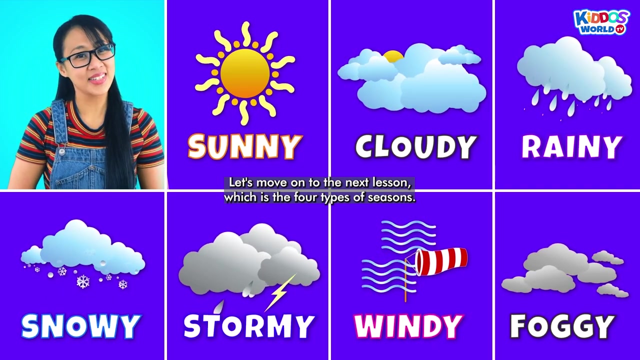 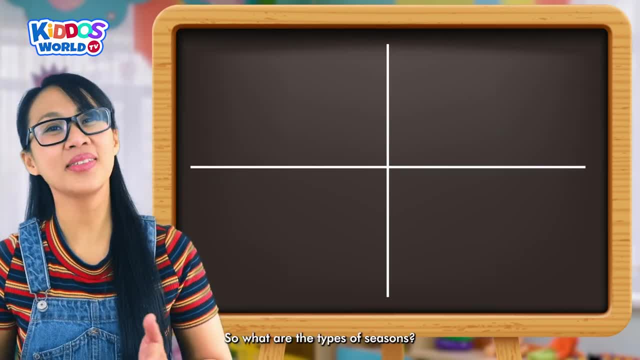 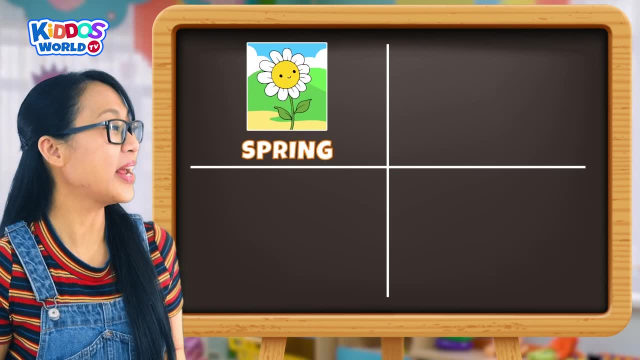 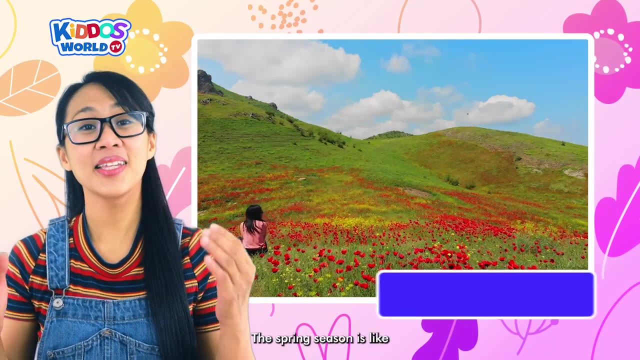 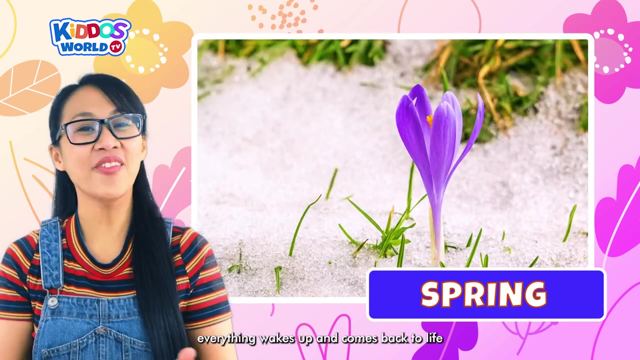 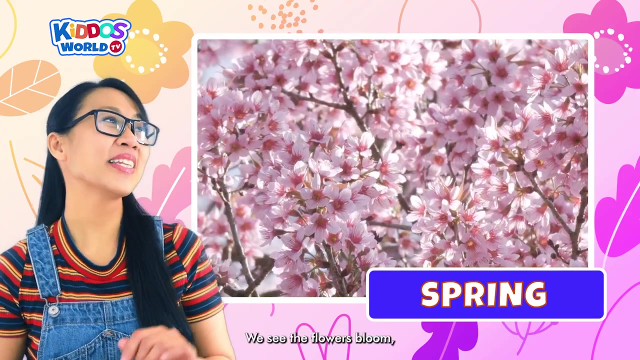 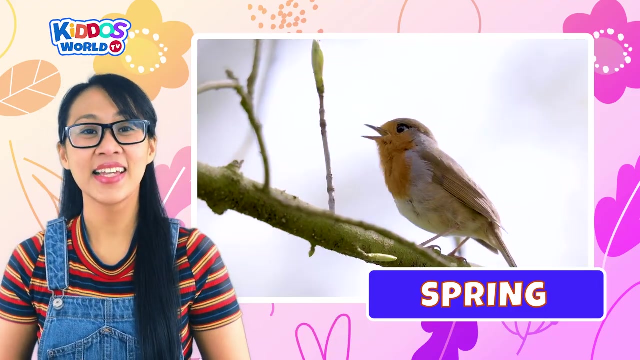 Love it. So what are the types of seasons? Let's tackle the first one, Spring. The spring season is like nature's birthday party. In this happy season, everything wakes up and comes back to life after a long winter. We see the flowers bloom, the leaves change and the birds sing again. 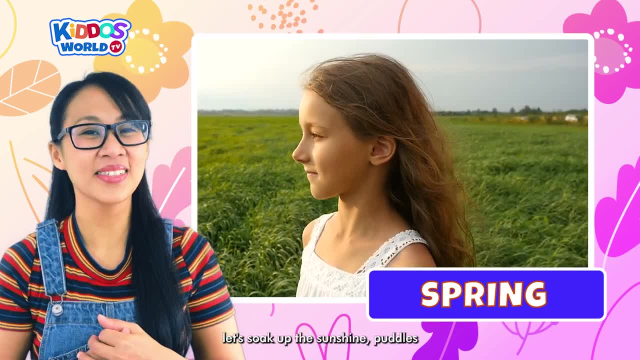 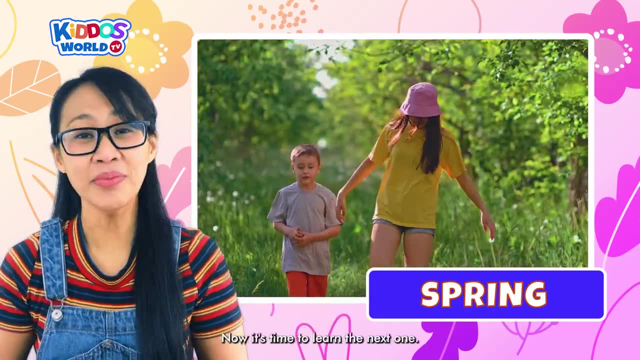 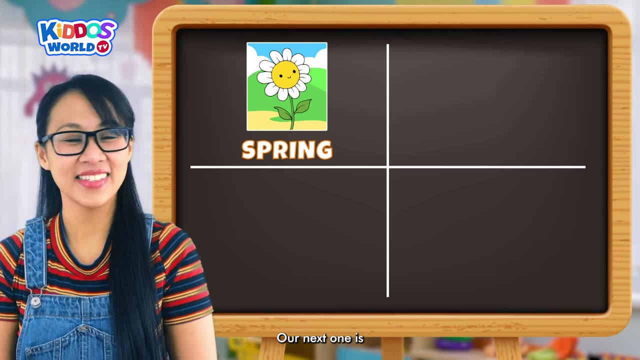 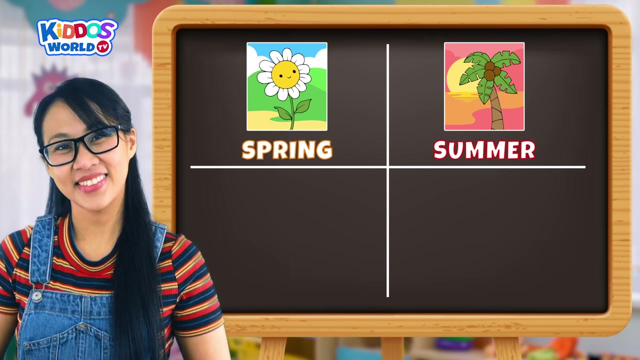 Now that spring has sprung, let's soak up the sunshine, puddles and all the new life that spring brings. Now it's time to learn. the next one: Fantastic. Our next one is Summer. Yay, Summer, Marvelous. Summer is like a big, long vacation. 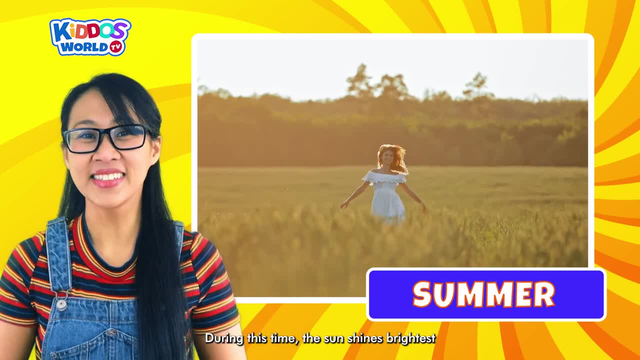 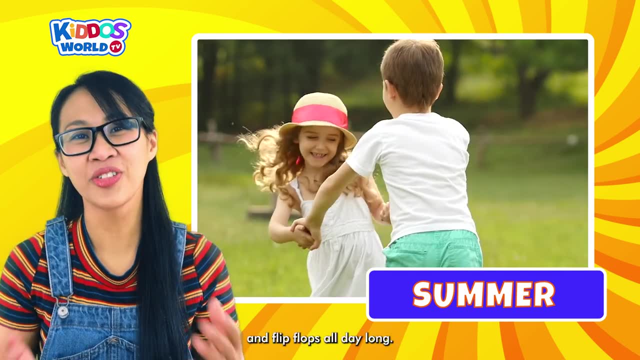 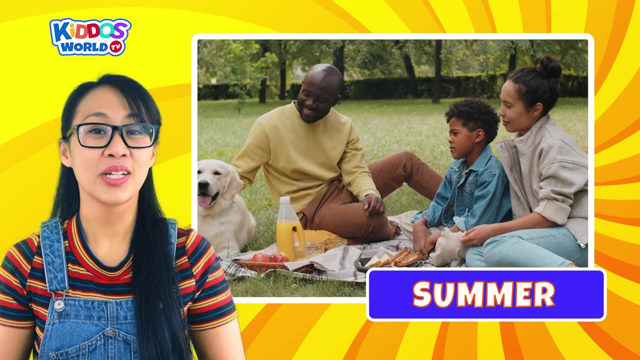 During this time, the sun shines brightest and the air feels warm and cozy. The weather is just perfect for wearing shorts and flip-flops. all day long, You can have picnics with your family and friends, swim in the pool and eat ice cream. 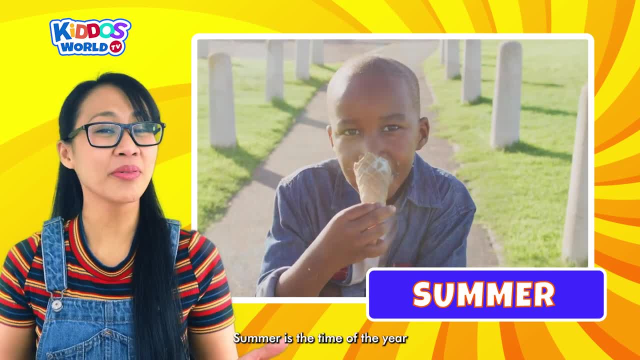 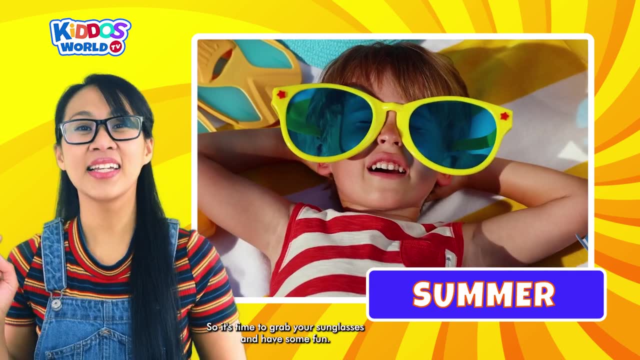 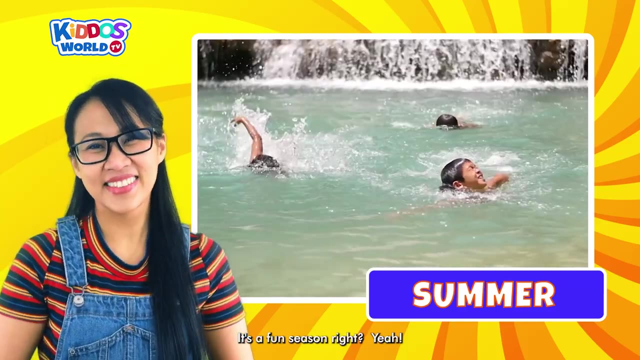 Woohoo. Summer is the time of the year when we take a break from school and have lots of fun in the sun, So it's time to grab your sunglasses and have some fun. It's a fun season, right Yeah? 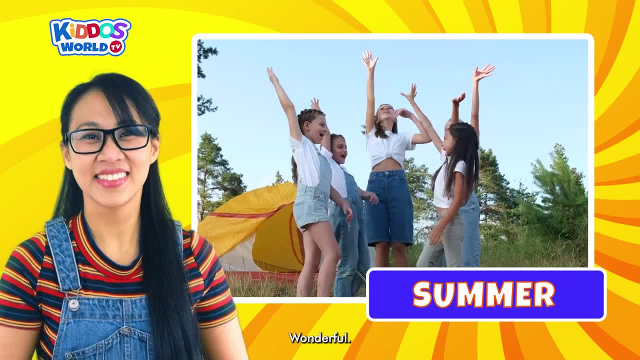 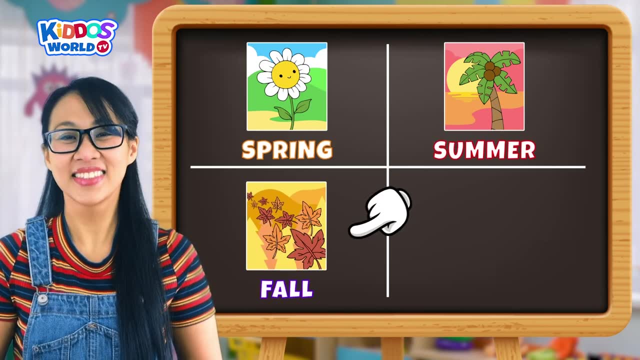 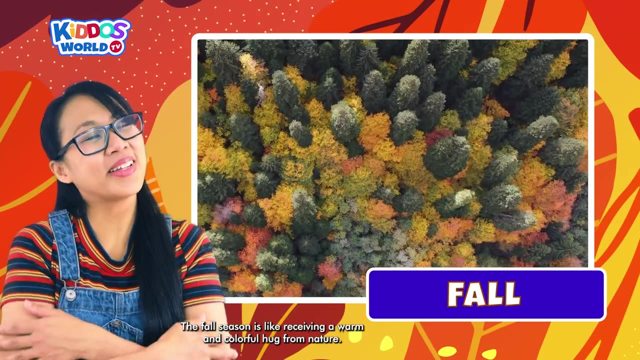 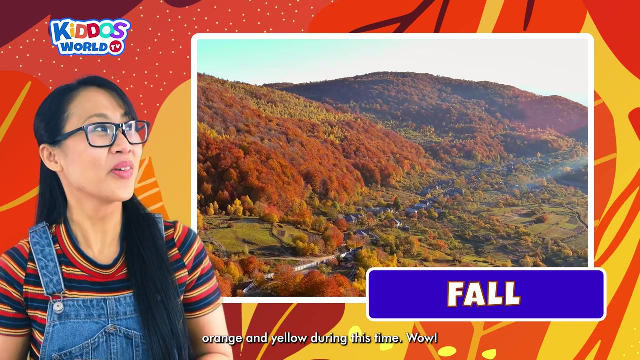 Now let's move on to the next season. Wonderful, Our next season is Fall. Fall, The fall season- is like receiving a warm and colorful hug from nature. The leaves on the trees turn beautiful shades of red, orange and yellow during this time. 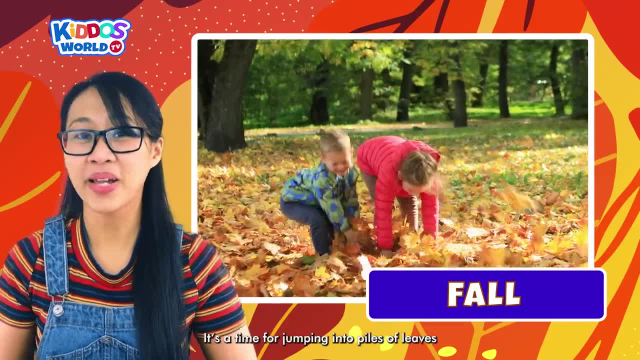 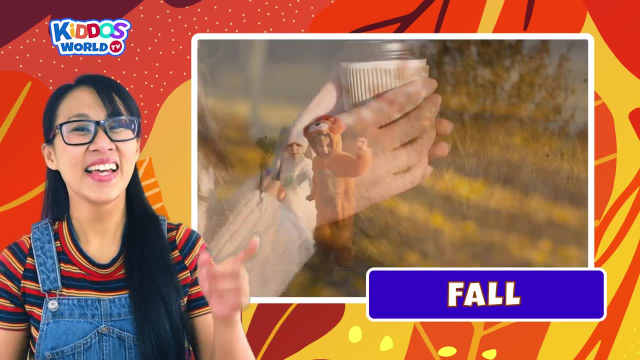 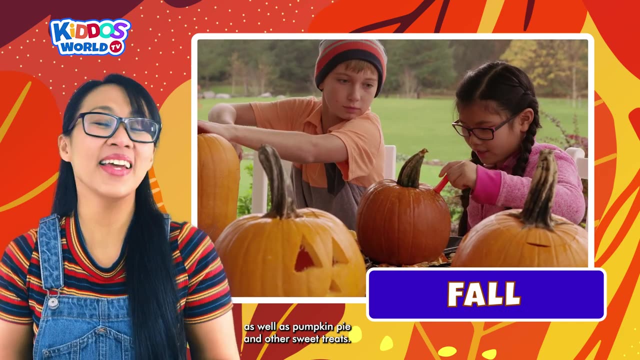 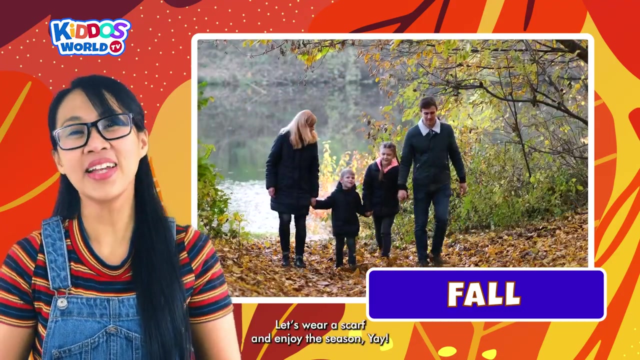 Wow, It's a time for jumping into piles of leaves, wearing cozy sweaters and sipping hot chocolate. Halloween and Thanksgiving are also celebrated in the fall, as well as pumpkin pie and other sweet treats. Now the fall is here, let's wear a scarf and enjoy the season.